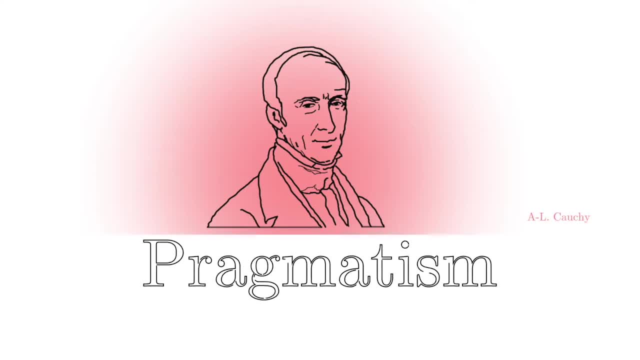 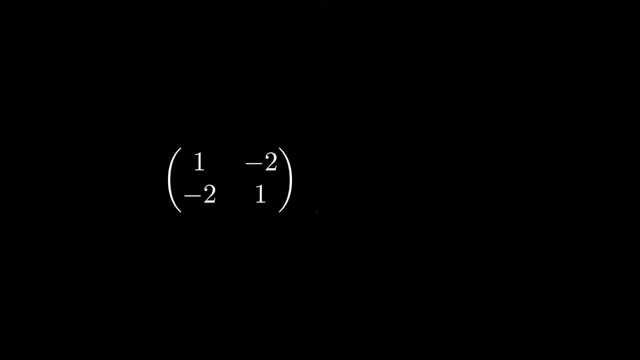 Why is this weird matrix product defined that way? Is it possible to interpret it? Yes, Today I'm going to show you how to visualize geometrically matrices. This will make algebra much more intuitive for you. In fact, you will be much more comfortable finding eigenvalues and eigenvectors. 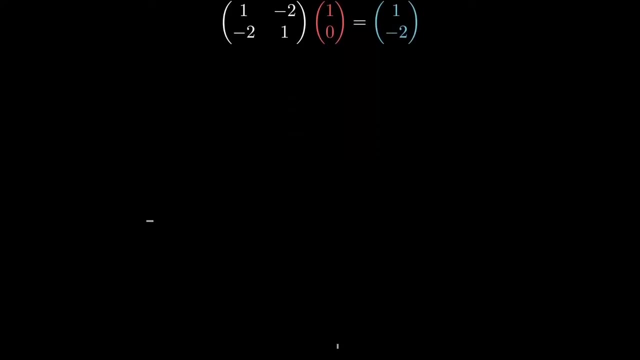 and matrix calculation will be easier for you. So stay focused, let's go. I considered a 2x2 matrix to show you quickly that the geometric interpretation of matrices boils down to plotting the vectors of the standard basis of the plane or the 3D space. 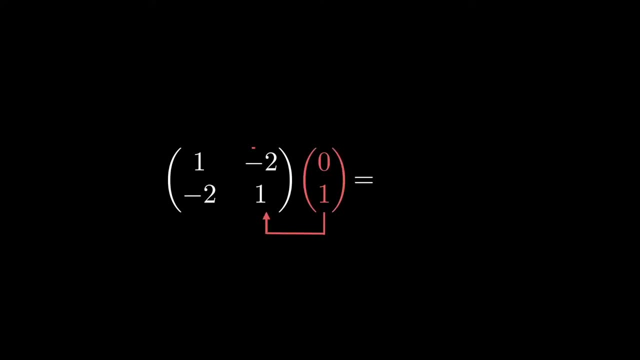 if you want to visualize a 3x3 matrix and what we will call their respective images, by the matrix considered, That is, each of the vectors written, when we multiply each of the vectors of the standard basis by the matrix considered, In order to understand the principle on which this geometric interpretation is based, I'd 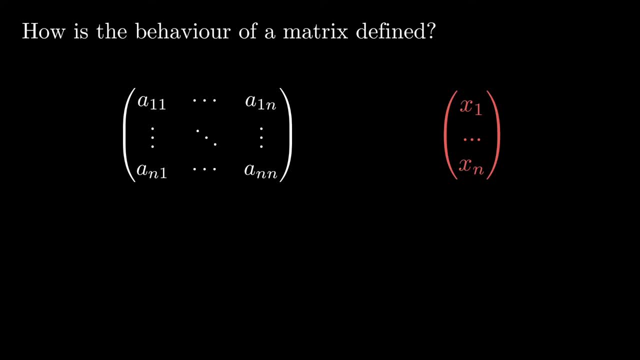 like firstly to define what is called the behavior of a matrix, to show you that a matrix is quite similar to a function that takes a vector in a certain vector space and returns another vector in the same vector space. We will call the vector returned by a matrix. 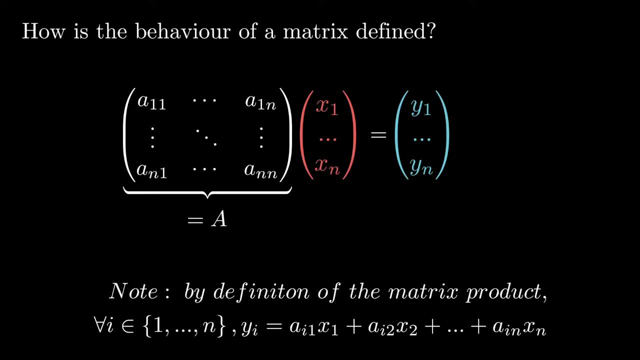 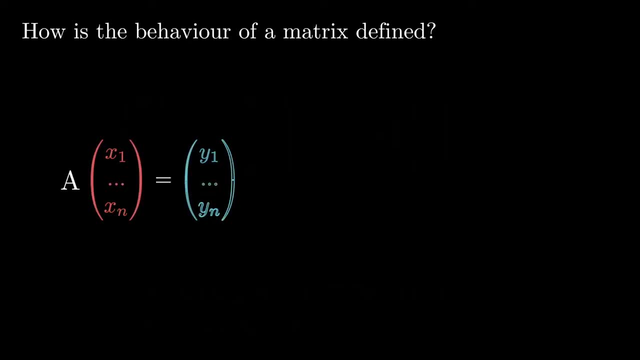 when this matrix is multiplied by another vector, an image vector, For instance. we can see what happens after we multiply each of the vectors which are equivalents to a vector in a given matrix. I proved the following equivalence in a previous video: where F is the endomorphism. 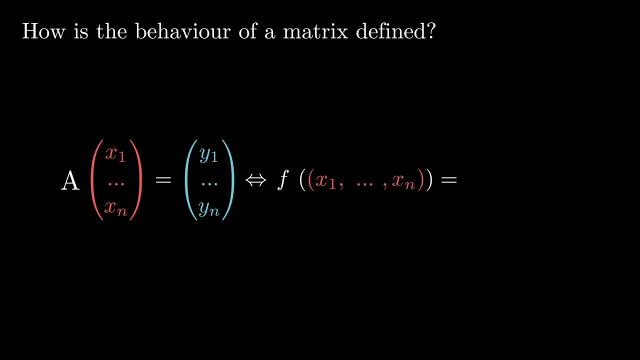 canadaically associated with the matrix A. If you didn't see this video, that's not a problem, but I recommend that you see it to have a better understanding of how an endomorphism is associated with a matrix. You can find the link in the description. 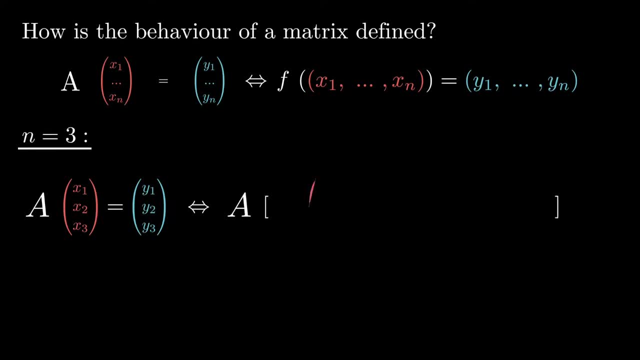 Let's now consider a 3x3 matrix For a 2x2 matrix. it's the exact same result. You can see through this equality that in order to determine the behavior of a matrix, we just have to derive the product of the matrix and each. 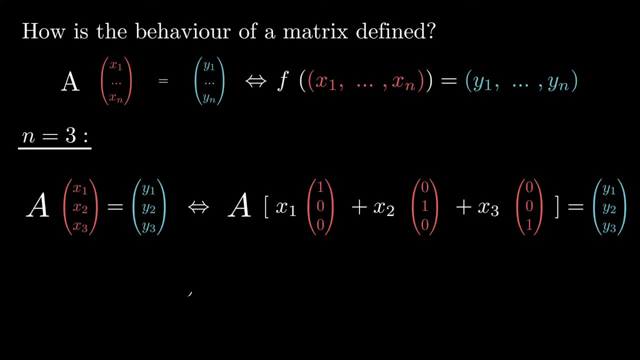 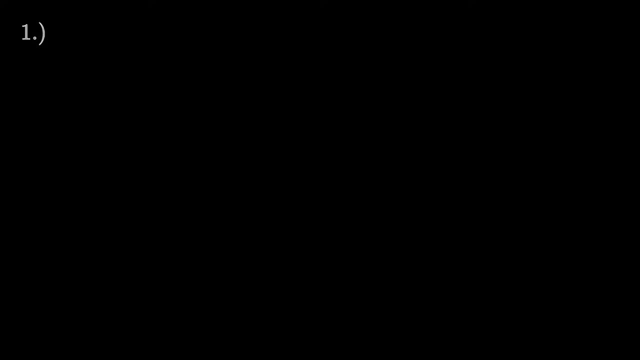 of the vectors of the canonical basis. To do so, I advise you to keep in mind the following: When a matrix is multiplied by the i-th canonical vector, where i is between 1 and the size of the matrix, the result must be equal to the i-th column of the matrix. 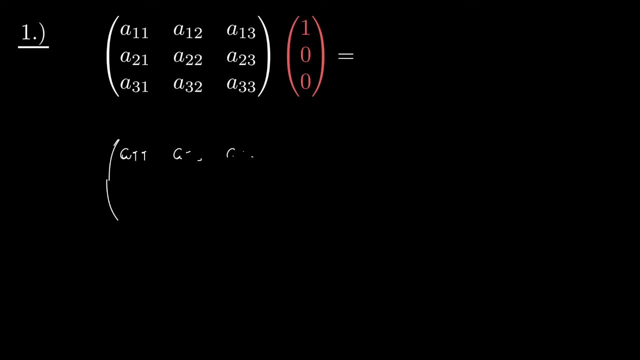 You could simply derive it by using the definition of the matrix product, but it's much more convenient to say it like this, especially when you want to visualize geometrically matrices. For instance, when this 3x3 matrix is multiplied by the vector, which is the first. 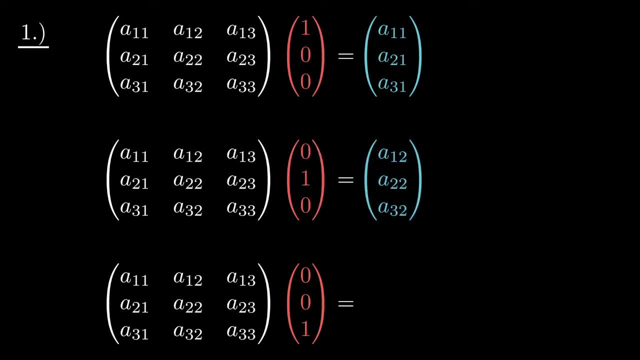 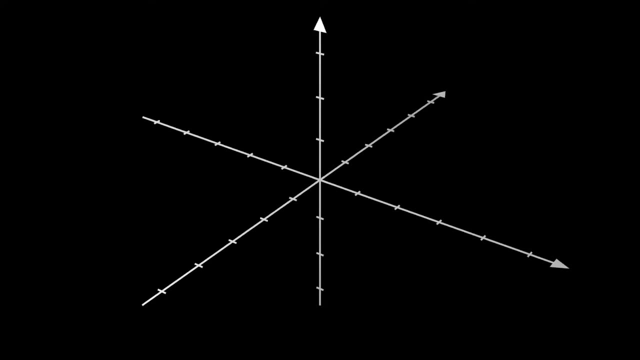 canonical vector of the 3D space, the product must be equal to the first column of the matrix. To come back to the interpretation process, when you finish plotting the 6 vectors in this case, or the 4 vectors in 2D, you have to focus on the image vectors of each of the 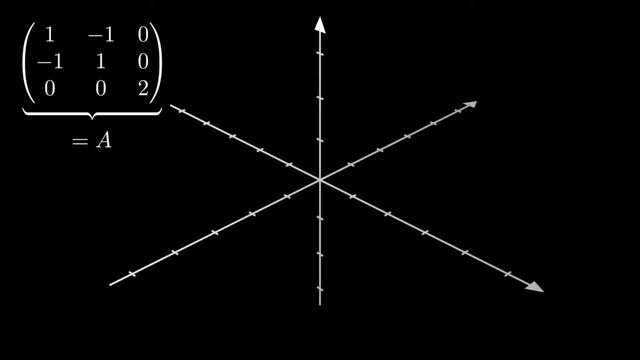 vectors of the standard basis. I plotted them in blue here. If one of these image vectors is collinear to its empty scene vector, then you've got to do the following: The first image vector is a vector of the matrix found, an eigenvector and therefore an eigenvalue. 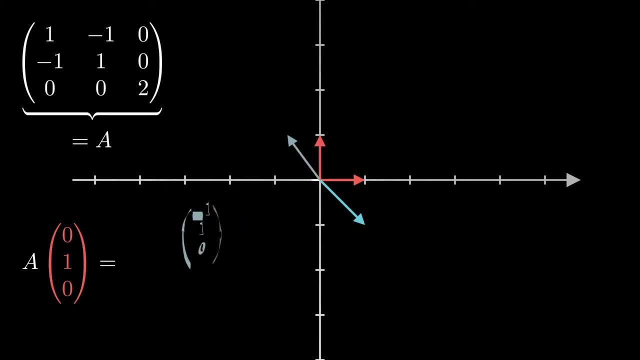 If two of these special and matched vectors are collinear, then you can find a linear combination of the two corresponding antecedent vectors, Such that this linear combination is an eigenvector corresponding to the eigenvalue 0. And this linear combination is a linear combination of the two corresponding antecedent vectors.